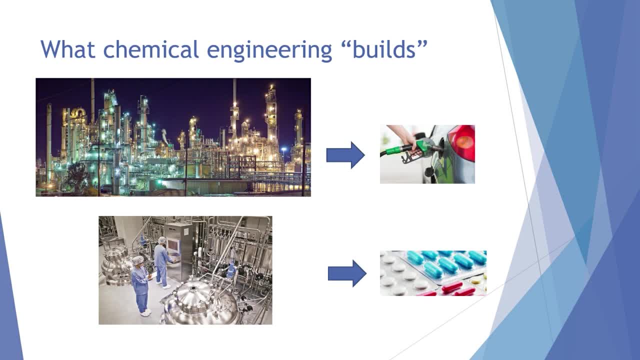 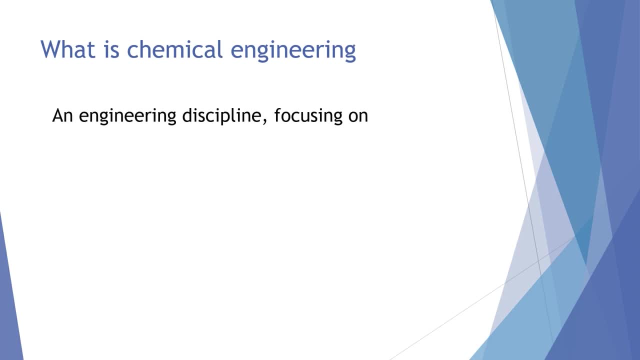 So we have seen what chemical engineering makes and what it builds. but what is chemical engineering? I would say it is an engineering discipline which focuses on transport and transformation of materials, accompanied with the transport and transformation of energy. And what makes chemical engineering really special is that we do these things on materials and energy primarily at molecular level. 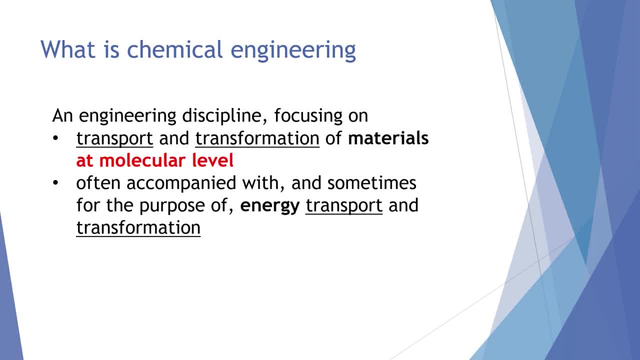 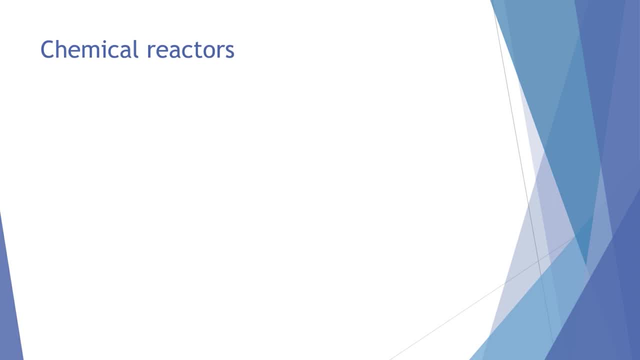 And which marks a key difference from, for example, civil engineering or mechanical engineering. Okay, so at the core of chemical engineering is a concept of reactors, And we have different types of reactors if you start with the conventional chemical reactors. and we have different types of reactors if you start with the conventional chemical reactors. 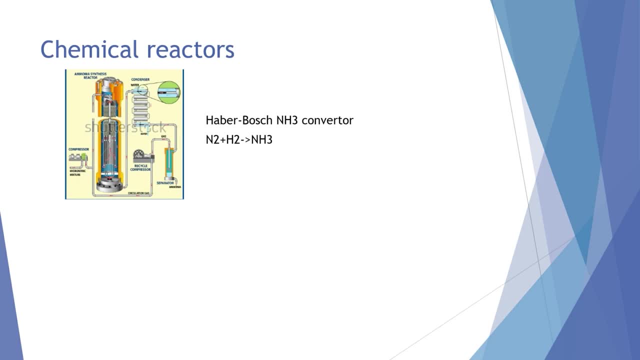 so here I have got an example which is the Haber-Bosch converter for producing ammonia, fluorine, nitrogen and hydrogen. so here I have got an example which is the Haber-Bosch converter for producing ammonia, fluorine, nitrogen and hydrogen. 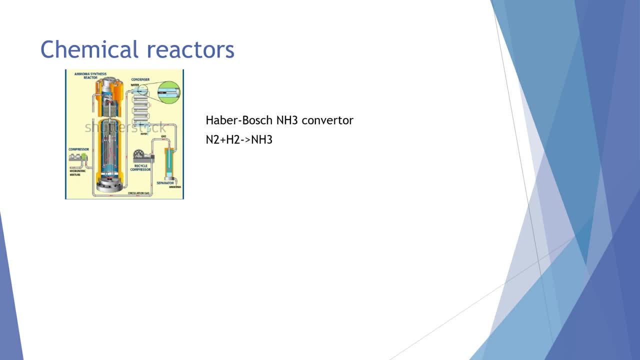 I put it up here because Akikon-ショi toys can get a lot of energy from this stuff, one of the earliest reactor designs operating at high temperature and high pressure, with catalyst So, and the other one I show here is the something taken. 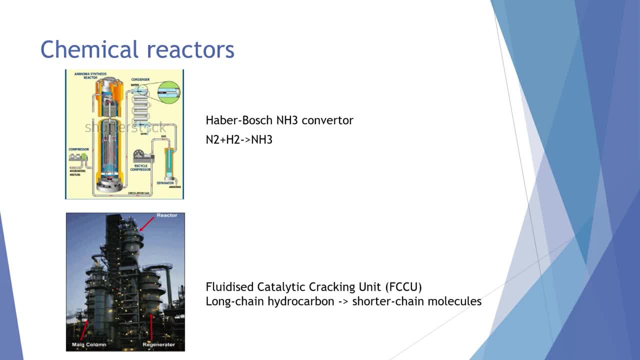 from oil refinery is a fluidized catalytic cracking unit, or FCCU, which is for producing short chain molecules from long chain hydrocarbon. So the reason why I put up these two reactors is because they do carry some historical importance. If you look at Haber-Bosch reactors for making ammonia, 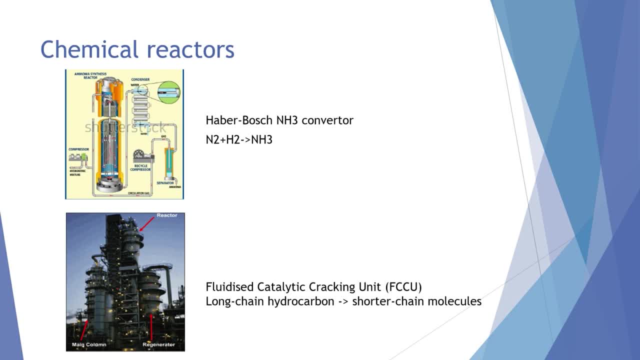 and many people believe is that this kind of chemical synthesis of ammonia, enabled by the Haber-Bosch process, has played a very important role in a food production, because ammonia is a major fertilizer and this has been very important for sustaining food production. So this is a good example of a fuel supply for the growing world population. 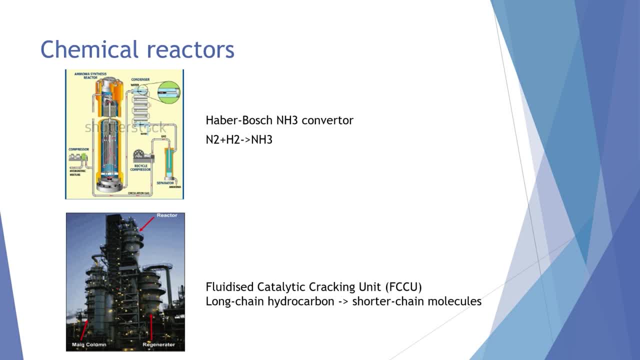 And what about FCCU? People who are familiar with the history of Second World War might have seen a statement about the importance of the fuels produced by this technology in the victory of the British and US Air Force, because of the the supply of high quality fuels required for for the air forces. so but 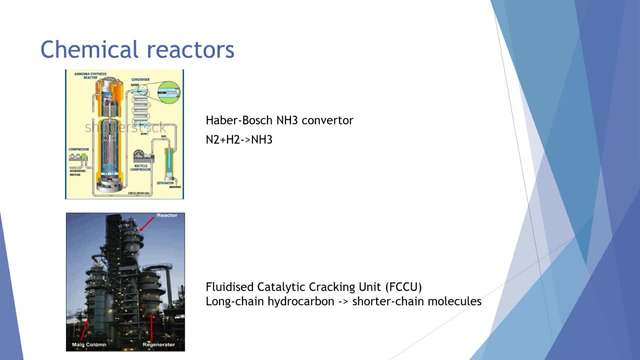 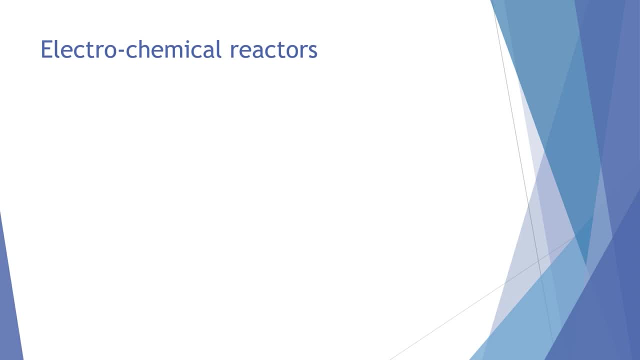 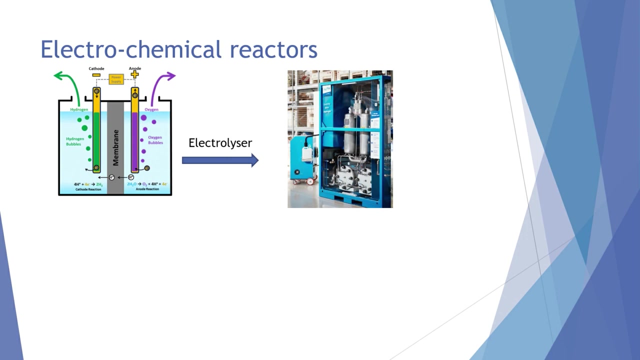 of course, reactors are not just chemical reactors. there are other times so, for example, electrochemical reactors which would involve the conversion between chemical and electricity, and this includes electrolysis, which converts electricity into chemicals, and fuel cells which go the other way around, converting chemical energy into electrical power. and these kind of 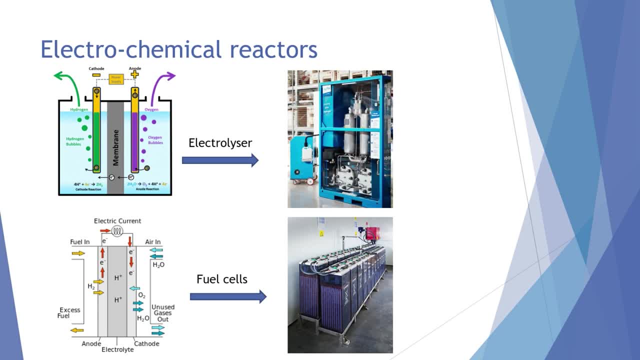 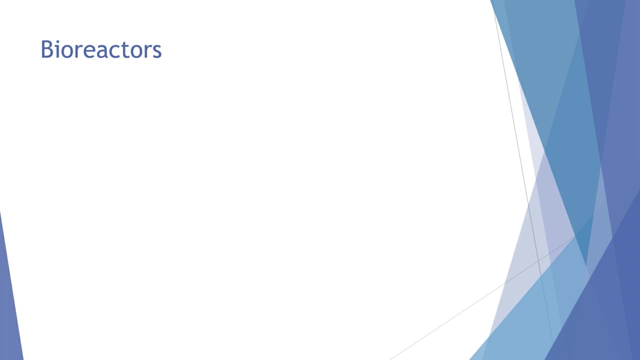 reactors are becoming increasingly important in the context of generation and utilization of renewable energy and clean energy. so then we have these bioreactors. it's a very important type of reactors. here I have example of a fermenter, and some of you might know that a key microorganisms used by a fermenter is a yeast, and if you zoom in, 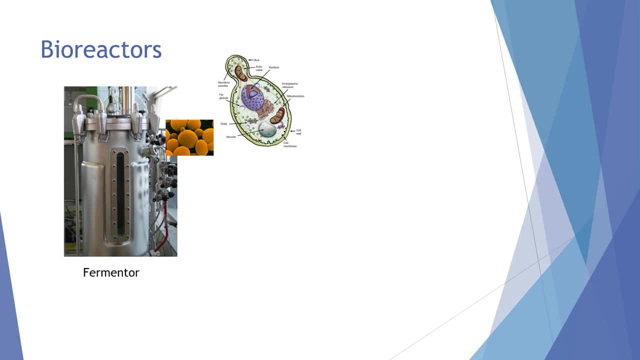 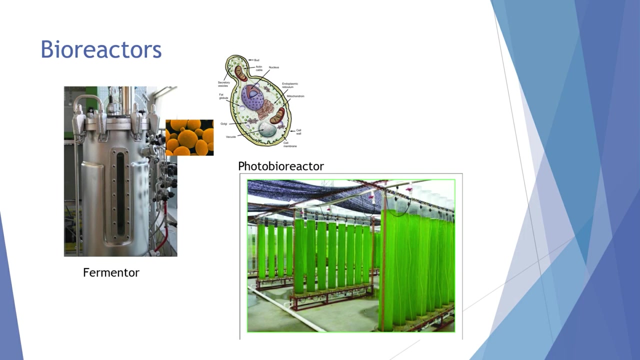 you can see, within these cells you have a complex biological machineries which can be used to convert substrate like sugar into valuable products like alcohol, through fermentation processes. and another example is a photobioreactor where microalgae is cultured. so these are unicellular microorganisms, again with a interesting set of bio. 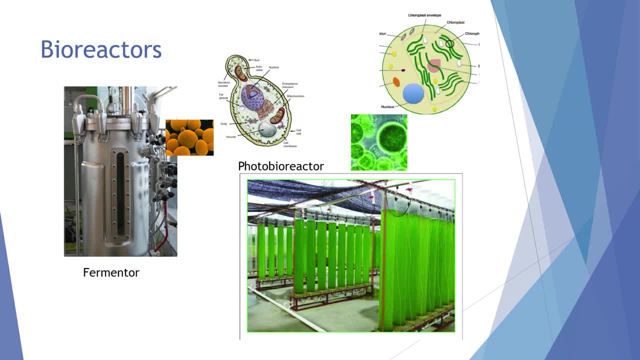 machineries which can convert CO2 into biomass through photosynthesis, and then the biomass can in turn be converted to useful products. so, but of course there are many other examples of bioreactors. I'm not showing more examples here, but just to say that this biochemical engineering branch of 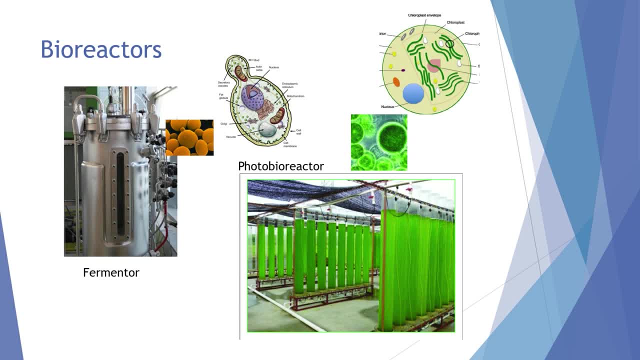 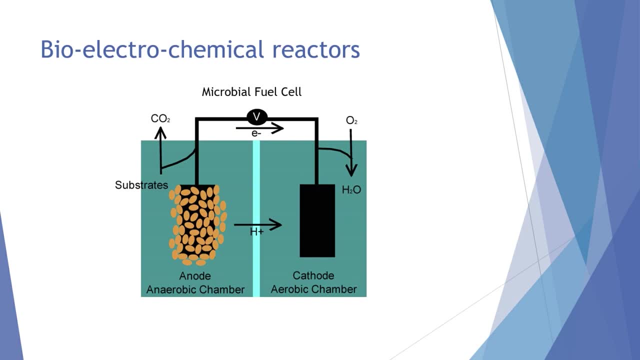 chemical engineering is becoming more and more important in many areas. so just to make things a bit more complex now, we can even have a little bit of question here about the ontology part of this presentation. what are some of the types of bioelectronics we have in the innovation? 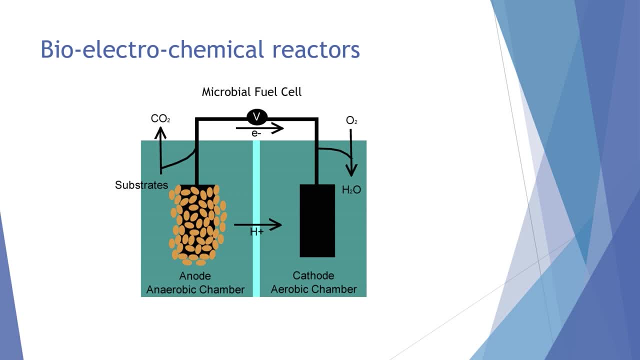 process. I guess the main thing is a single cell reactor which combines the bioelectrical and chemical. so example here is a microbial fuel cell where you have microorganisms in the anode chamber of the reactor converting substrate into electricity which can be, for example, applied in recovering the energy. 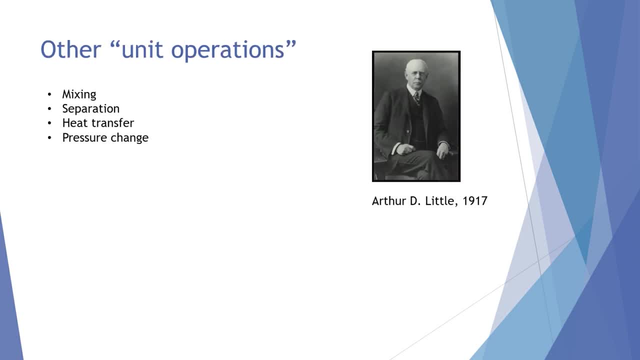 from wastewater. But the operation of reactors will need to be supported by some other so-called unit operations, such as for mixing, separation, heat transfer and pressure change. And in fact the concept of unit operations was formed in early 20th centuries by pioneering. 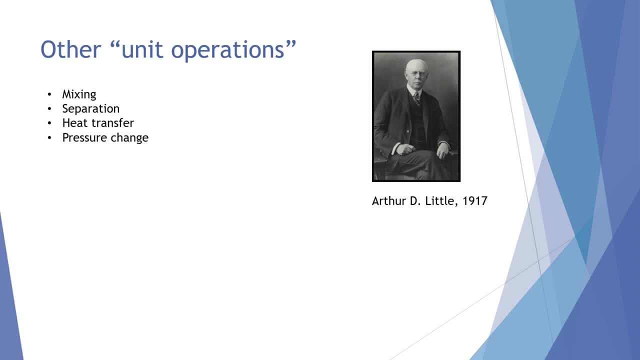 chemical engineers such as Professor Arthur Litter, and the formation of this concept of unit operations somehow marked the birth of modern chemical engineering. So I have an example here. if you have taken GCSE or A-level chemistry, you would recognize what this is. it's a distillation device. you might have played with it in your lab. 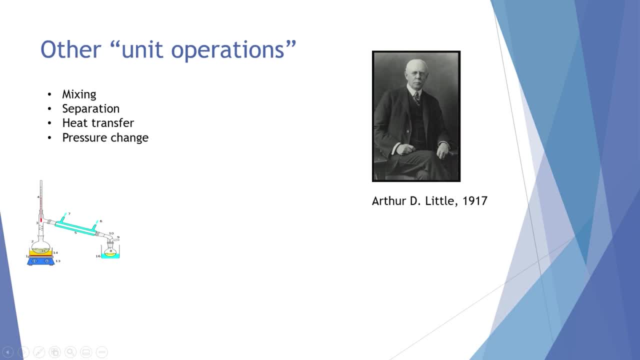 in your high school And this, you know, is linked to a key separation unit operations. Okay, So it's a distillation column. so in chemical engineering we do something very similar to what you have seen here, but just in a kind of bigger, larger scale. 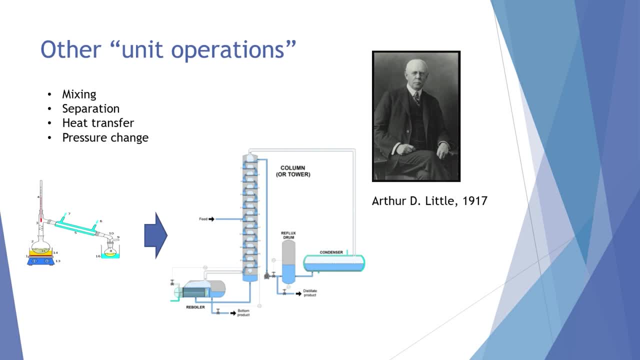 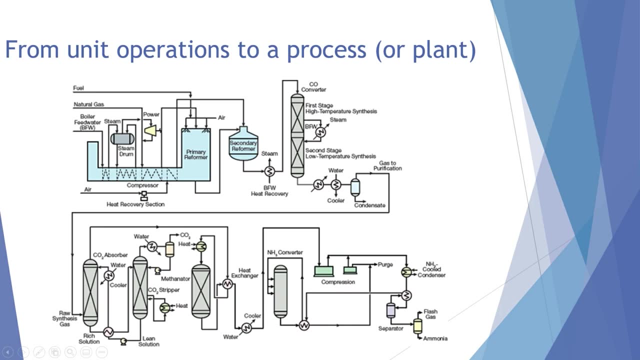 So we have seen reactors and unit operations, but one complexity of chemical engineering is that we have to link these different unit operations to form a whole process, a whole plant. So I think the example shown here is again a little bit more complicated. 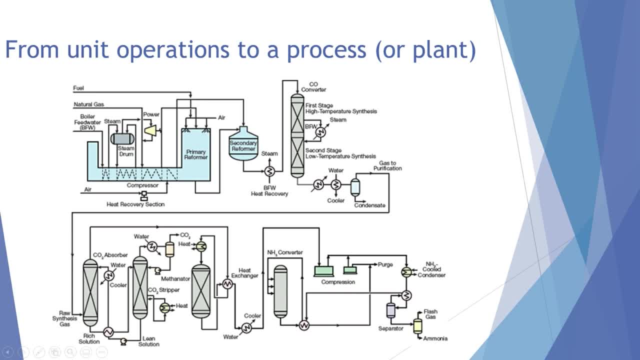 Okay, So this is again ammonia production. So this is the Haber-Bosch reactor we have seen earlier on, but you can see as a whole ammonia plant. it's much more complex than just the reactor alone, right? 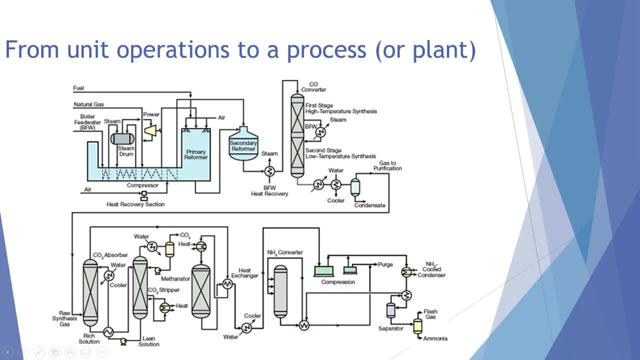 You have the. here you have the reforming of natural gas for the conversion of CO2, conversion of carbon monoxide into CO2 and hydrogen. Okay, So here is the removal of CO2, and then you have the. finally, the ammonia synthesis with. 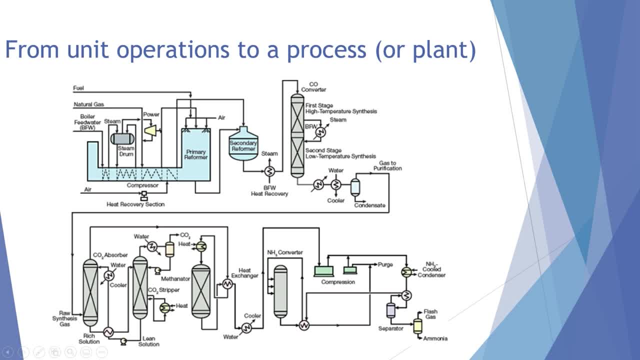 hydrogen and the nitrogen, and here you have the separation of ammonia product. As you can see, for the whole plant to work properly, you need to have the unit operations to operate in unison, if you wish, so that we can run, you know, a productive and stable 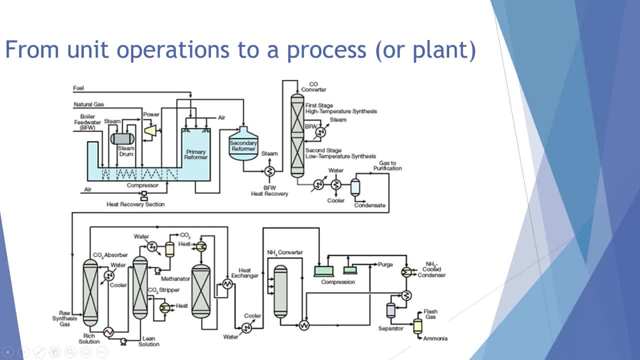 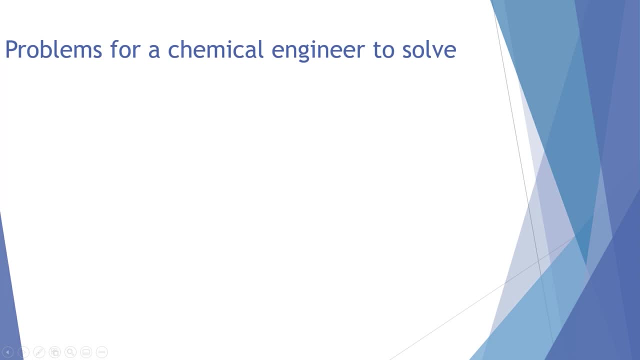 process. So the design and operation of such a complex process certainly requires a lot of thinking, a lot of careful design, a lot of careful decision-making. So what are the problems, then, a chemical engineer is expected to solve in their daily life? Well, I'm sure this list wouldn't really surprise you, based on what we have seen earlier. so 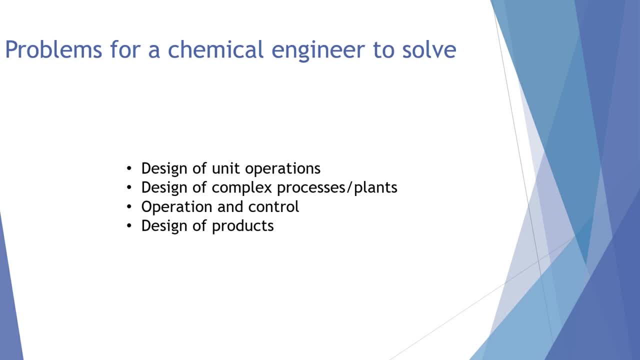 we have the design of unit operations, design of the complex process of plants, looking after operation and control, and also design of products. So, but how would we judge whether we have done a good job on any one of these? Well, we need to look at a number of objectives. 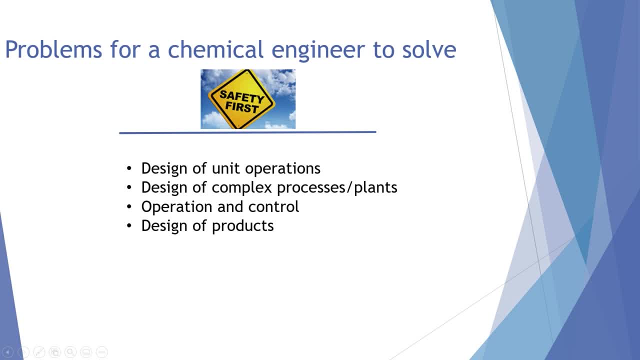 So, whatever we do, we have to ensure safety. Safety is always the most important thing- Okay Well, for any engineering, but particularly for chemical engineering, and we always try to improve the efficiency of materials and energy and to make things implemented in. 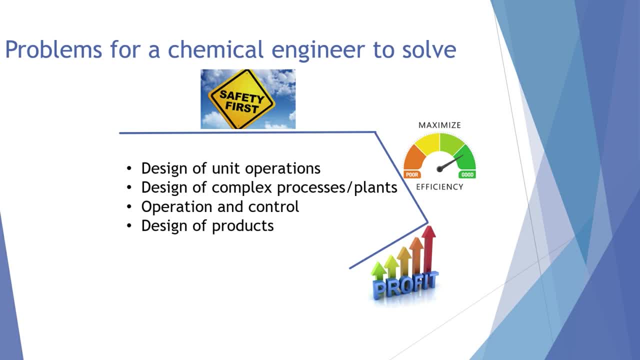 the industry. it has to be profitable, so it should have a good economics, and we do need to look after our environment And as well as the social sustainability. So you can see we have multiple objectives, which means the chemical engineering is really. 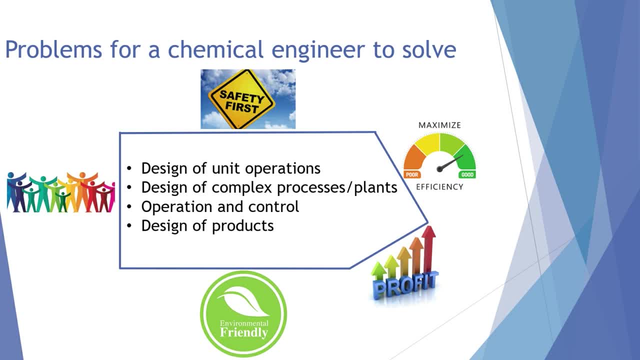 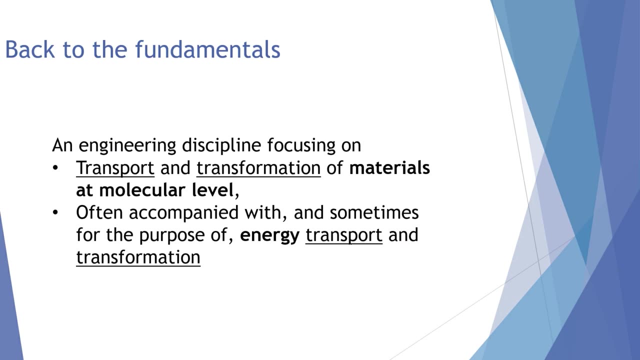 a very, very demanding job. So how we can make our students capable of handling such complex jobs? Well, this has to be done. you know, we come back to the fundamentals. This has to be done. Okay, This has to be done by going through a rigorous training. 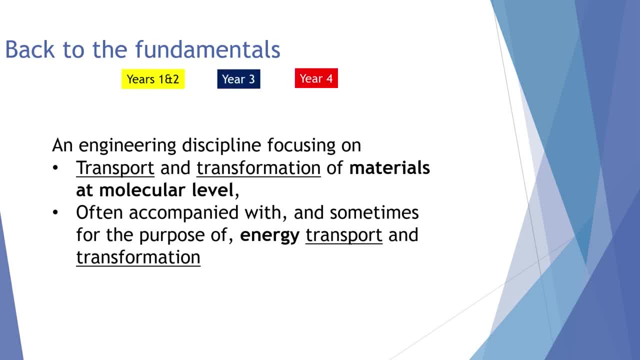 So in Oxford in this department, if you look at a four-year program going from the first two years with common engineering training and then into the third year and the fourth year where students can get a bit more specialized in one or several areas, so the students will 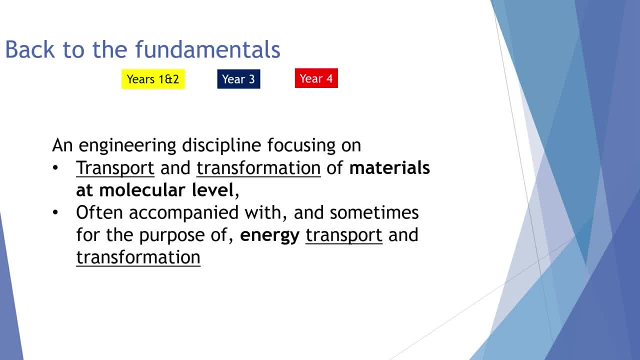 be taking a number of courses Which would address all the important aspects of chemical engineering, either on the- you know, the material side or on the energy side. So these are the specific courses, but don't forget that in year one and year two there 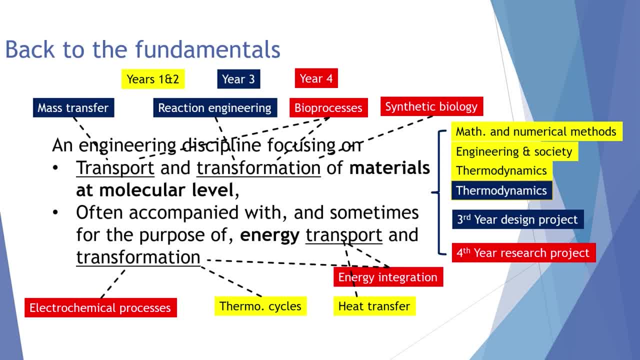 are common courses in mathematics and numerical methods, engineering and society, and also thermodynamics, Which are Which are useful for all the engineering disciplines, but of course they are also very, very important for chemical engineering. And then, moving on to year three, thermodynamics will be learned further, which forms a very 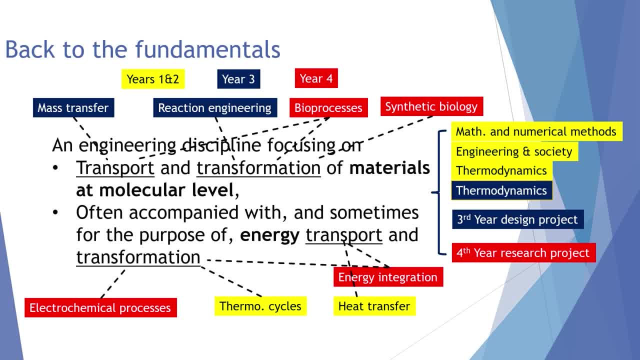 important foundation for many aspects of chemical engineering. In addition to these different courses, we do have two major projects throughout the four-year program. So in the third year there will be a design project. This is a group-based activity, So at the moment we're running a design project with our third year student in the 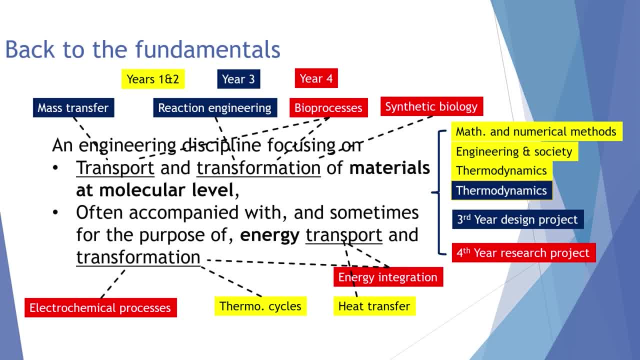 area of carbon capture and utilization, And particularly it is about designing a chemical plant which can turn CO2 into methanol. So it's very interesting topic. And then in the fourth year there will be individual research projects, projects and every year there are a number of chemical engineering oriented research. 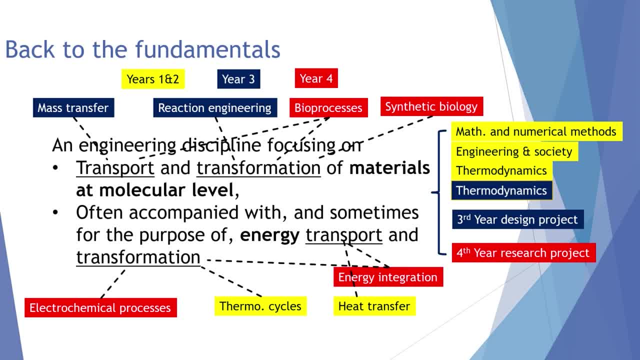 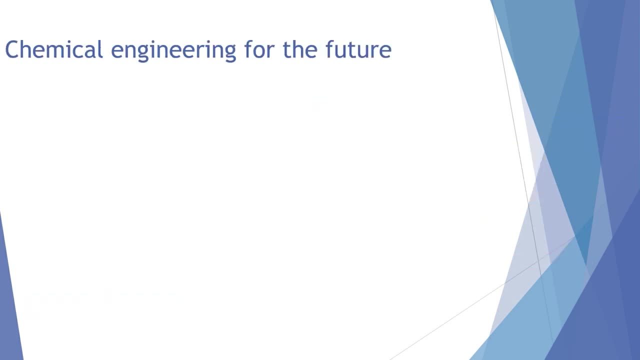 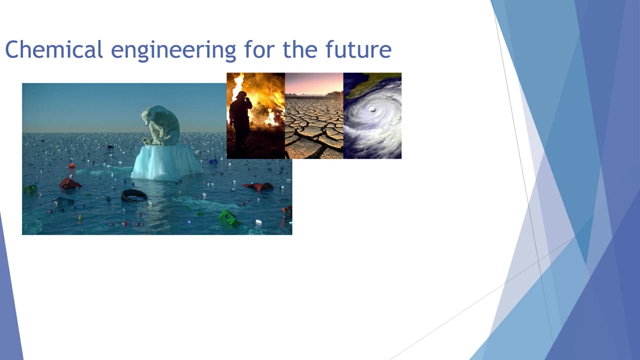 projects offered to our students. So these courses and projects will, we believe, get our students well equipped for the chemical engineering career. but they will be educated not only for to become the workforce today, but rather to prepare them to meet the demand of future challenges. So, and here I guess we can, you know, look at a major challenge. 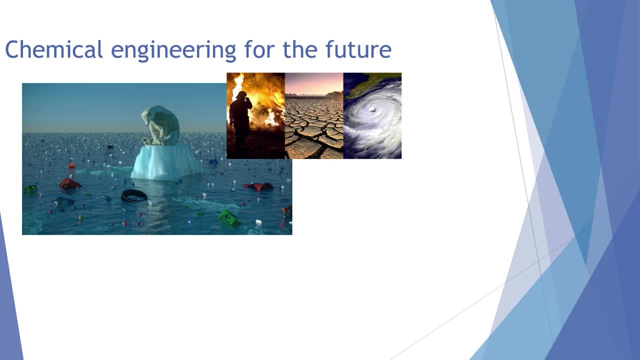 from climate change is, I guess, widely recognized as a major challenge for our society in the future. and in the UK, for example, we also face an aging population and which points to the challenges in the future. health: So we have environmental health, we have human health, and chemical engineering should certainly make a great contribution. 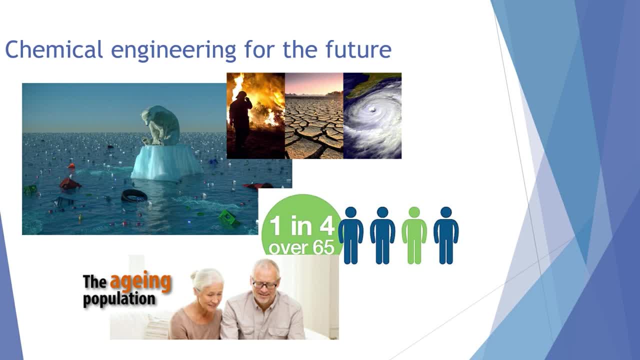 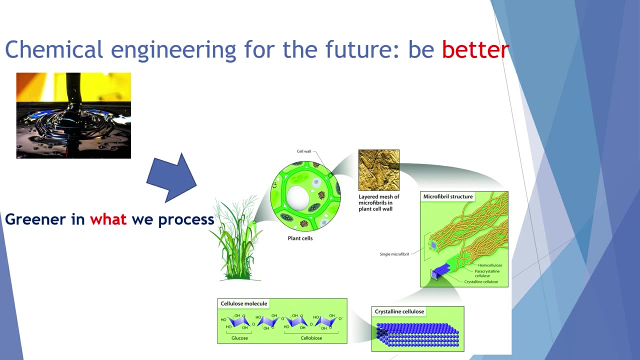 to address the future challenges in both areas. So how we do that? Well, I guess there are two different things we can do. One is for the products or services the chemical engineering is providing. now we can try to do them better, right? So the same products. 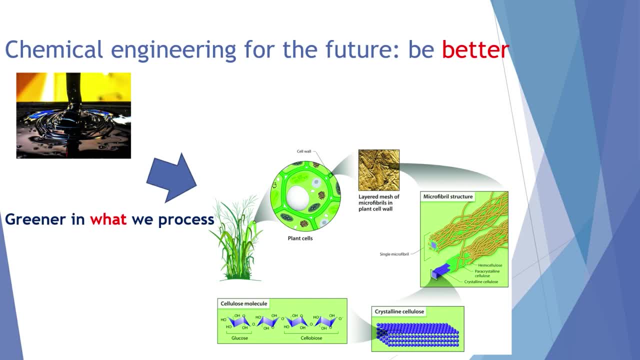 same services, but we try to do them better, For example, in order to produce certain chemicals or material. so instead of processing fossil resources, we try to make them better. We try to look at something greener to process, such as biomass. So, in the sense we can, 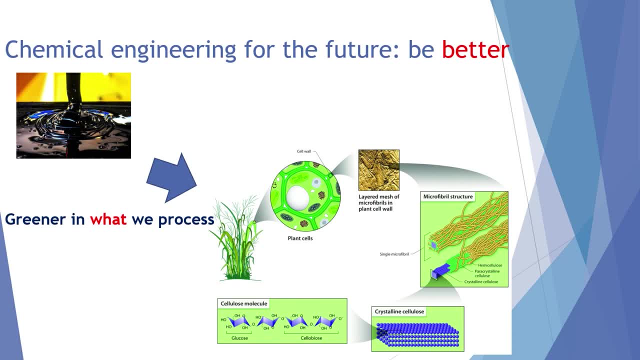 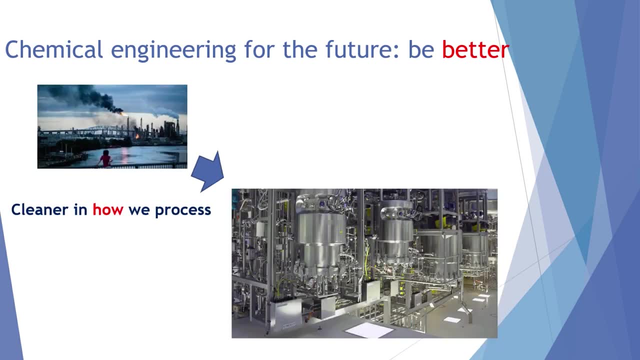 deliver the same chemicals and material, but by processing a different feed stock. Or we can be cleaner in how we process things, by reducing emissions- reducing energy consumption, water consumption, for example, but in a better way. Another thing that chemical engineering can do to meet the 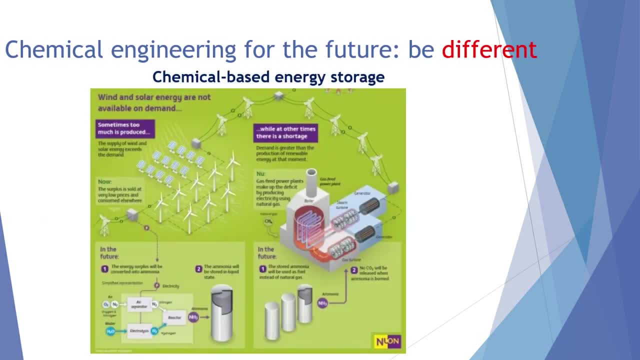 future challenges is to start offering something different from what we are offering now, And I have got a number of several examples taken from the research which is undertaken by our colleagues in chemical engineering here. So the first one shown here is a chemical based energy storage. So the 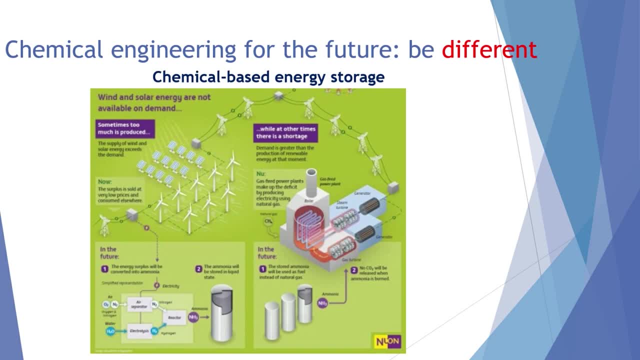 story here is we see the increasing penetration of renewable energy into the energy supply. One of the problems we have to face is that there is great intermittency or variability in what solar, of wind energy can can be made available to us. So one of the problems we have to face is that there is great inim cog勤 assist in real asset management. One of the problems we have to face is that there is greatreno cog勤. assist in real asset management On open veggie minus 12,000 세계 people with problems related to climate change, the global problems and environmental, or even the social blogs folder is longing to be an essential roll in order to be an stricter reader of the global economic boom. 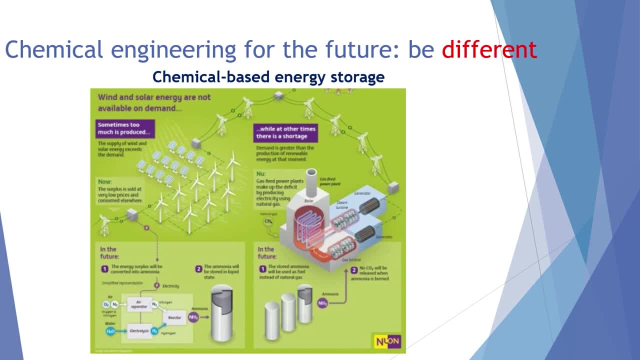 So how do we deal with this intermittency, or variability? Well, one of the approaches is by energy storage. So when there's a lot of energy available, we try to store it somehow, and then when there's deficit, we try to offer energy from the storage to meet the 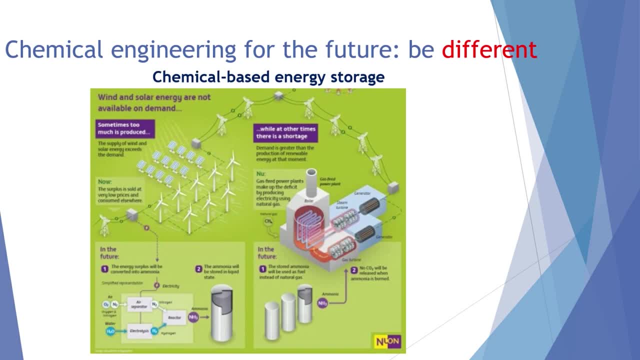 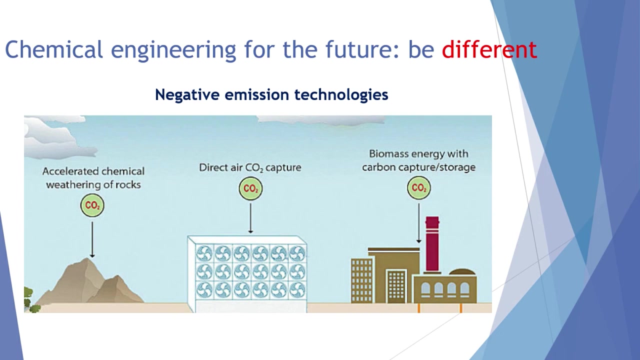 the demand, And chemical-based energy storage is one of the energy storage technologies and particularly useful for long-term storage and storage in a large volume or large quantity. So that is one area, And another area I show here is something called negative emission technologies. So this is about. 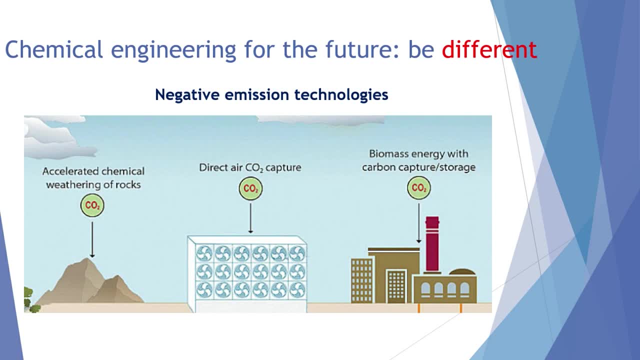 dealing with greenhouse gases. So we all know that we need to cut down the greenhouse gas emissions so that we don't get into very dangerous climate change, which is certainly true, very important, but many people believe that we might have already got too much greenhouse gas in the atmosphere. 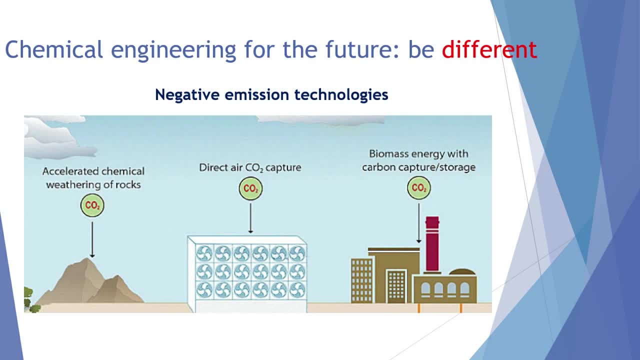 particularly CO2.. So the task of negative emission technologies is to take the CO2 which is already in the atmosphere out, And this can be done by different technologies and what is shown here. we have three things here. One is what is called accelerated weathering of rocks. 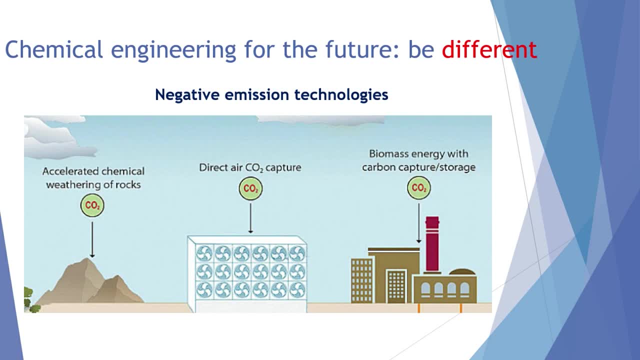 to promote the reaction between the CO2 in the air with the minerals, and this one is direct air capture. It's a kind of separation process. And here is the bioenergy, with carbon capture and storage. Basically, we grow trees, for example, and then we turn biomass into energy. 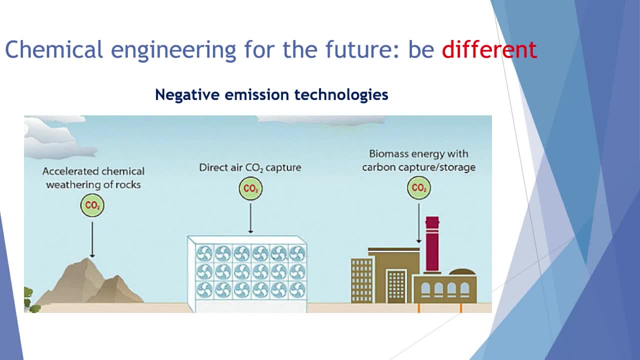 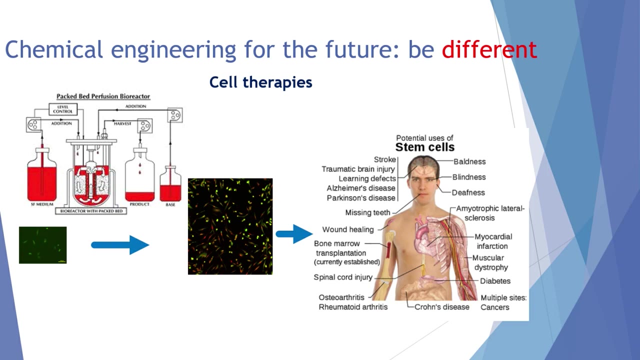 but in that kind of power conversion process we capture CO2 emitted And all of these you can see, they are very, very closely related to chemical engineering. And finally, so if we move from environmental challenges to human health challenges. so one example I show here. 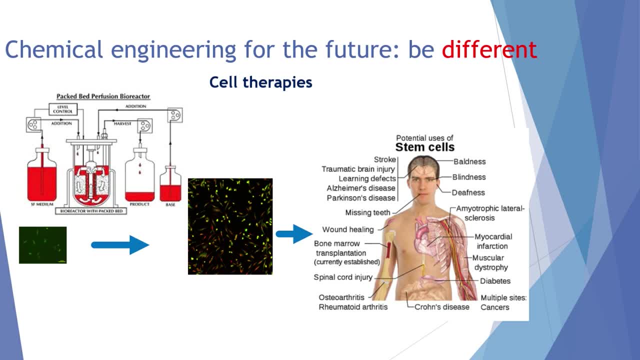 is about stem cells or cell therapies. So you might have heard of the good things that stem cells can do through cell therapies, but a fundamental requirement to do a cell therapy is that you need to have a sufficient amount of cells in good quality. So if you start with a rather limited number of cells, 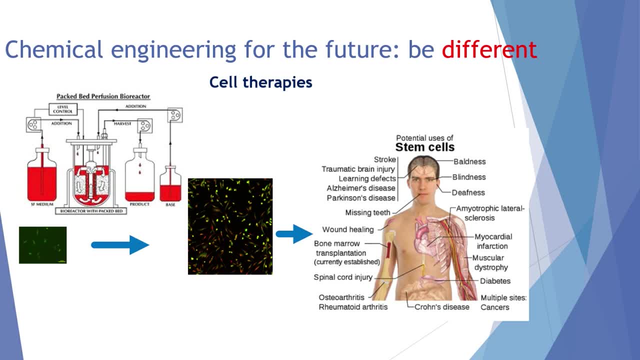 you definitely need to go through something called cell expansion And this can be done by kind of this biochemical engineering techniques, particularly biochemical bioreactor and which is capable of taking a small number of cells and to do the cells expansions to supply the cells. 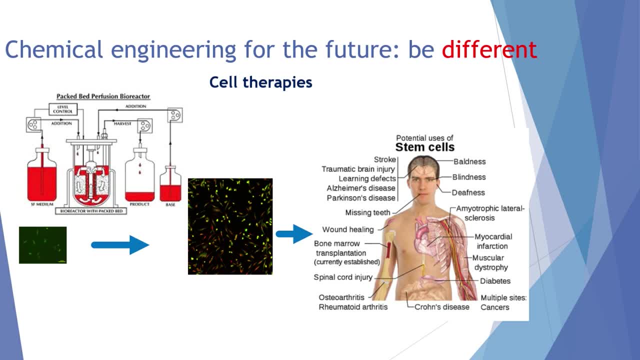 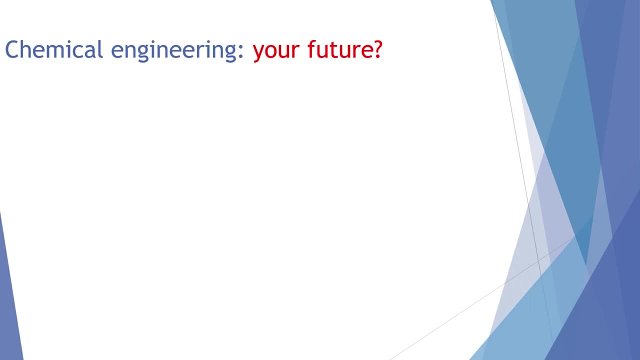 in the required quantity and required quality to enable cell therapies. So I think I'm coming to the. towards the end of this introduction. We talked about the chemical engineering futures and perhaps we can ask whether chemical engineering is your future. Well, I hope you know through this. 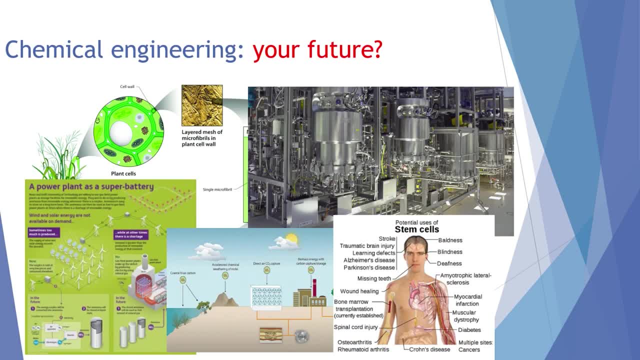 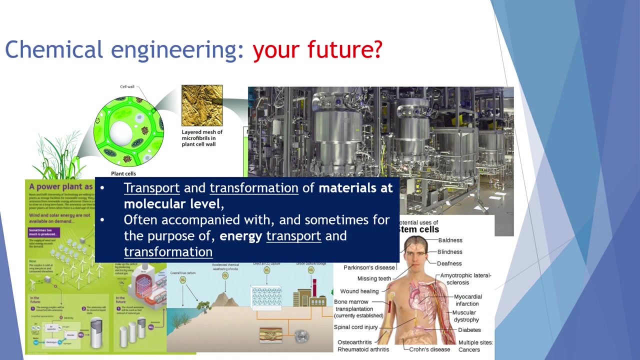 lecture you have seen some exciting future offering that chemical engineering can give to deal with future challenges ranging from the environmental side to the human health side, And I also hope that you feel some of the fundamentals of chemical engineering is interesting to you And, on top of this, if you are also.